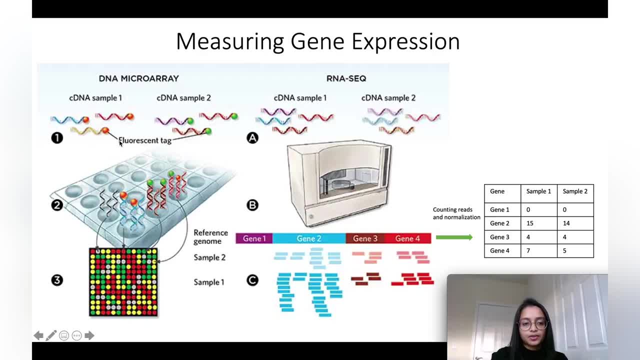 And these complementary DNA are labeled with fluorescent tags, Following which these complementary DNA are allowed to hybridize with probes. These probes are nothing but short DNA sequences that are complementary to the genes. In the following step, the plate is washed off and the unhybridized complementary DNA gets washed off. 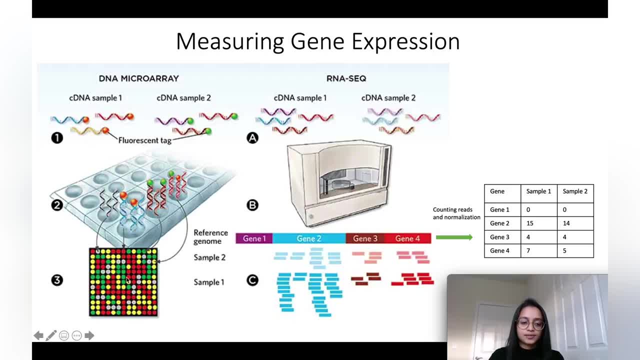 And what we get is a plate with different fluorescent intensities. Based on the fluorescent intensities, we can identify what genes are expressed in one sample or both the samples, or maybe differentially expressed between the samples. Talking about the RNA sequencing technology, mRNA from the samples are reverse transcribed. 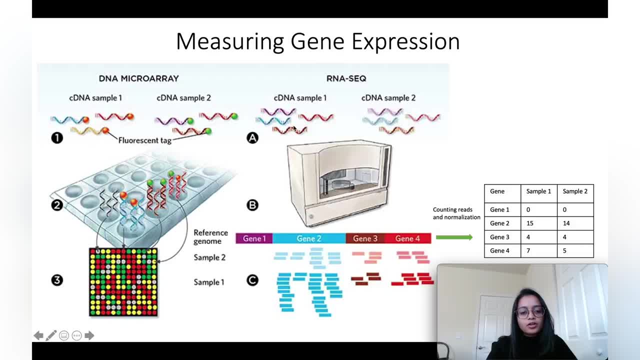 to complementary DNA. These complementary DNA are broken down into fragments and are fed into the DNA sequencer. The DNA sequencer gives out reads which are mapped to the reference genome. Based on the number of reads that are mapped to the reference genome, a gene quantification matrix or a count matrix is generated. 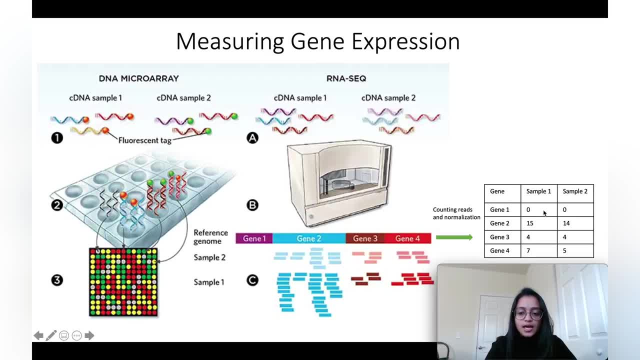 Essentially, the rows in the count matrix are genes and the columns are samples And the numbers correspond to the reads that map to the genome. To give you an example, we see that no reads from sample 1 and sample 2 map to gene 1.. 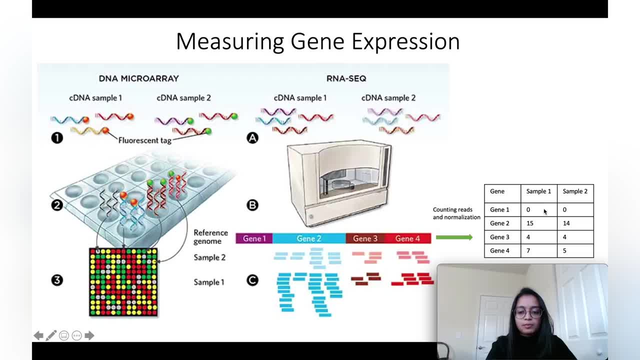 And hence we see the row corresponding to the gene 1 in sample 1 and sample 2 has zero. Similarly, there are some numbers of reads that map from sample 1 and sample 2 to gene 2. And hence the row corresponding to gene 2 from sample 1 and sample 2 have some numbers. 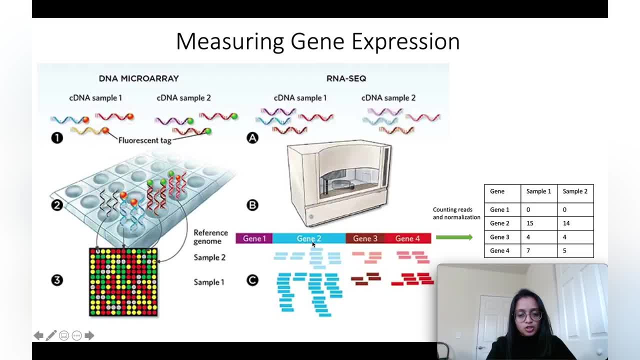 And these numbers are equivalent to the reads that map to gene 2 from the reference genome. Gene expression data can be in the form for count matrix or there can be some normalization or bias correction steps for the memorize or bias alt redo Reverse 영상 trong heterogen jewelry method. So 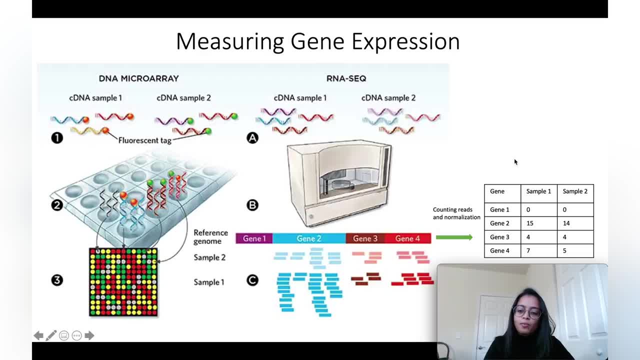 I am going to talk about genetic usage and therefore there areất to do sans MMAe reporters. in case of SocialUp, For the memory data of some of the hardware that are thought to be from sample 2, can be performed on this matrix. some common normalization methods are tpm, rpkm, fpkm or cpm. 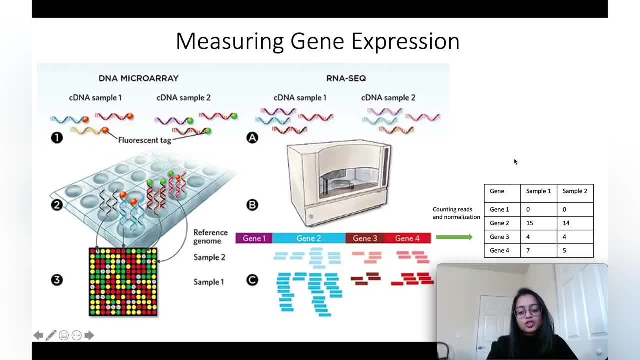 i will create a video in the future where i explain each of these normalization methods, but for the sake of our understanding, this is how a gene expression matrix, or a gene quantification matrix, is generated: based on the number of reads that are mapped to the genome. now that we have some understanding on how gene expression is measured, 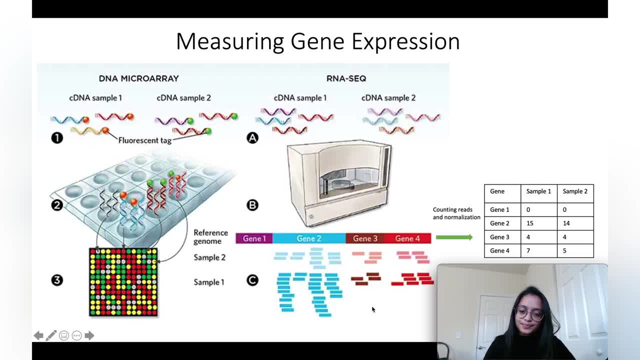 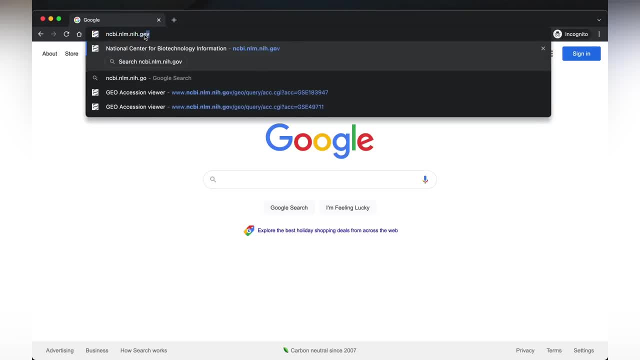 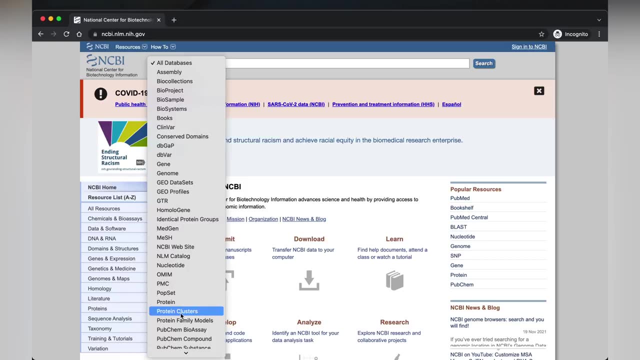 let's go to ncbi and start fetching our gene expression data. let's start by going on to the ncbinlmnihgov, the home page of ncbi, and this is what the home page looks like. here we have access to all the different types of databases present in ncbi. 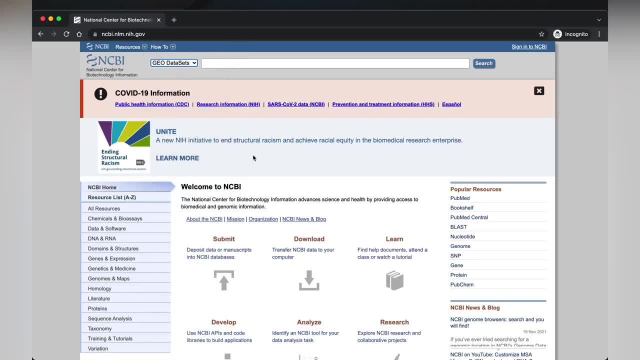 but today we are going to use geodt data sets. geo essentially stands for gene expression omnibus and since today we are interested in getting the gene expression data, this is the database that we will be utilizing today. there are two ways to search for data data sets in geo. either we can use the accession ids. 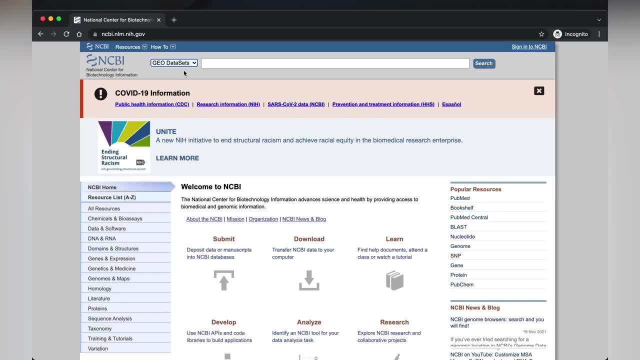 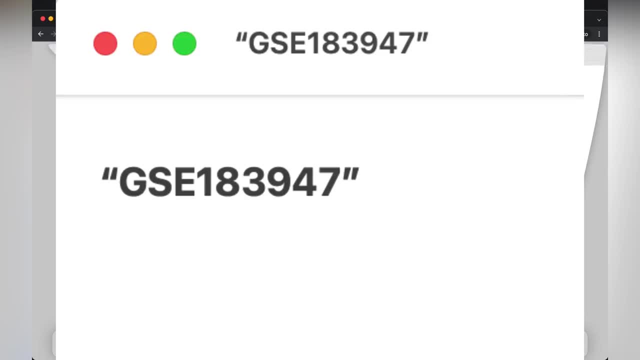 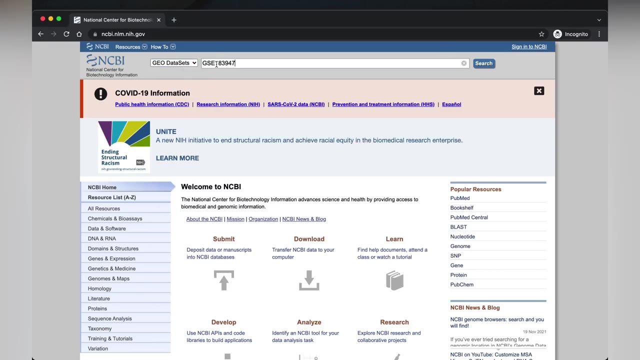 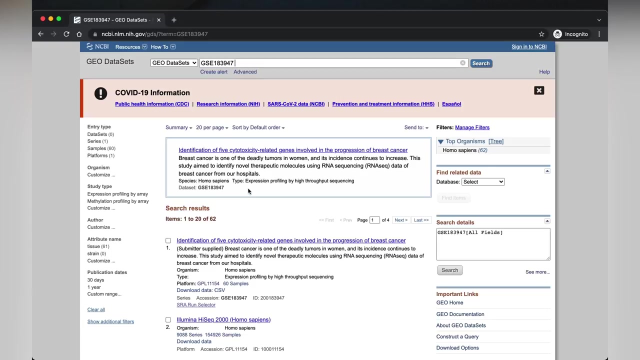 or we can use the keywords. each data set in the geo has a unique accession id. so today we are going to use an accession id that is gse183947 and we are going to click on search. this gse accession id is associated with the breast cancer data set. 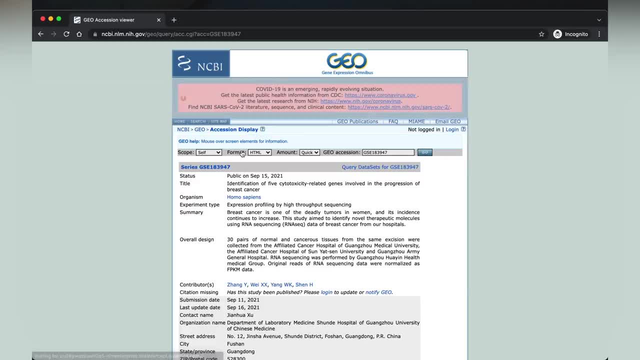 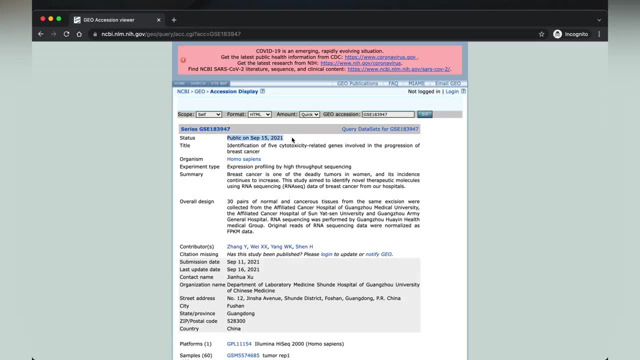 and the first hit that shows up, i'm going to click on that. this is what a gse record looks like. so here we have the status, which is the date when this data set was first made public. and it is the date when this data set was first made public and the title associated with the. 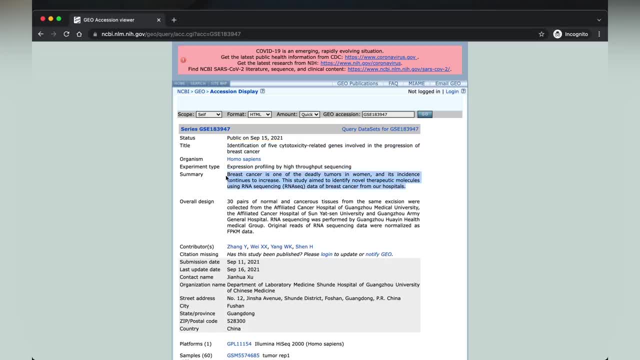 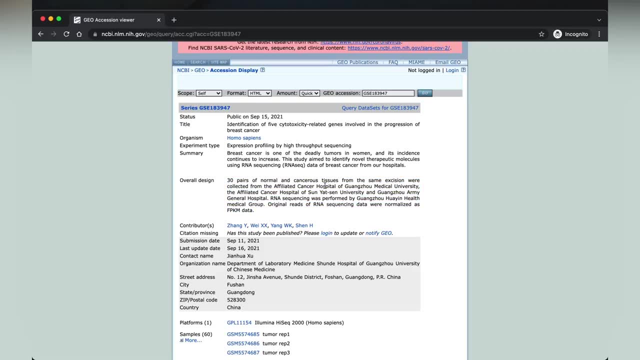 data set: the organism. the data set is derived from the experiment type and the summary. next we have the overall design, which tells us that the data set has 30 pairs of normal and cancerous tissues from the same accession, and rna sequencing was performed by this group. 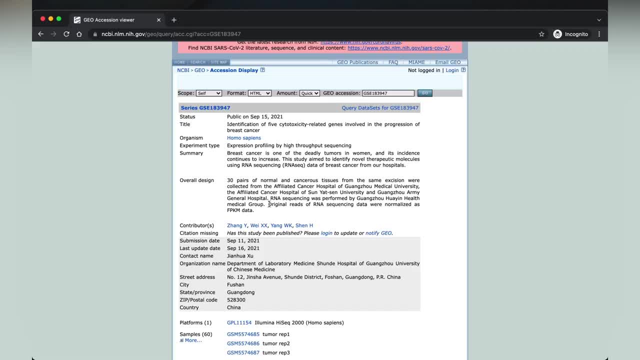 and the original reads of rna, sequencing data were normalized as fbkm. This sentence is a very important information to have when you're processing the data set. It is important to know what kind of normalization has been performed on your data set and it affects the conclusions that you draw from it. 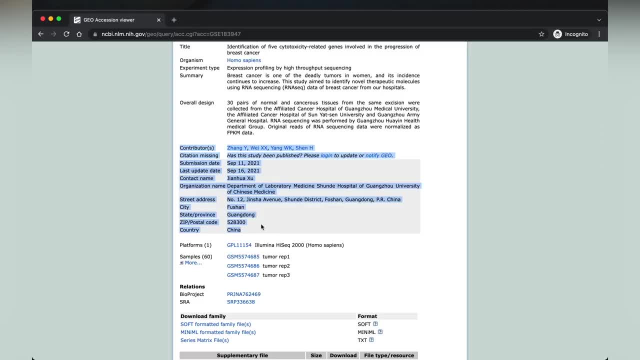 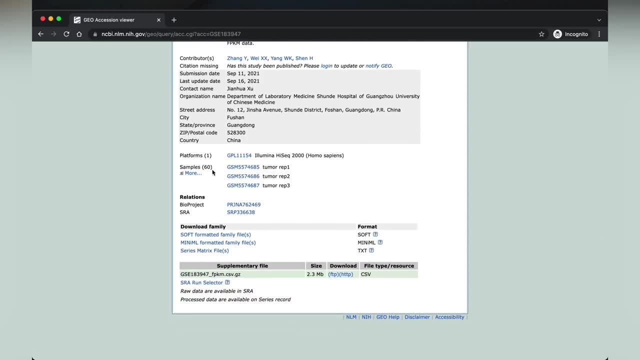 The section following, that is the information about the contributors of this data set. When we scroll down further, we see that we have sample information and we see that we have 60 samples. Since we have 30 pairs of tumor and normal, we expect the samples that should be 60. 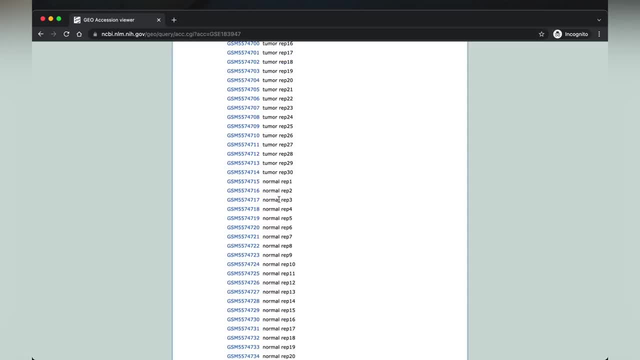 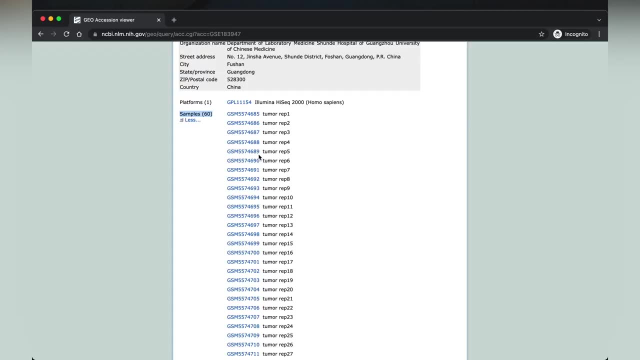 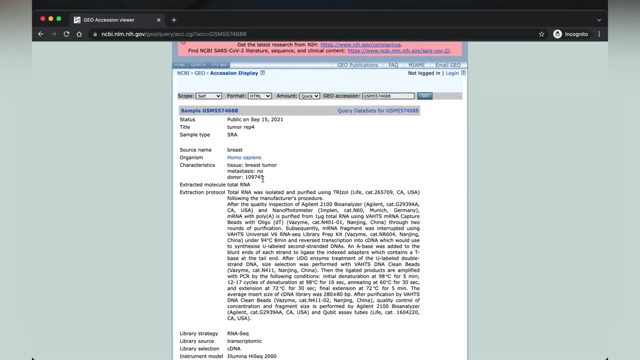 samples. You can click on more to take a look at all the samples here, and each sample here has a GSM ID associated with it. When you click on any one of the sample, you can get more information about the sample, more information about the characteristics, the extraction protocol and how. 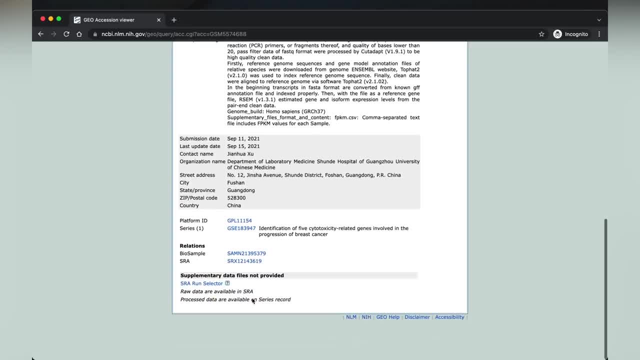 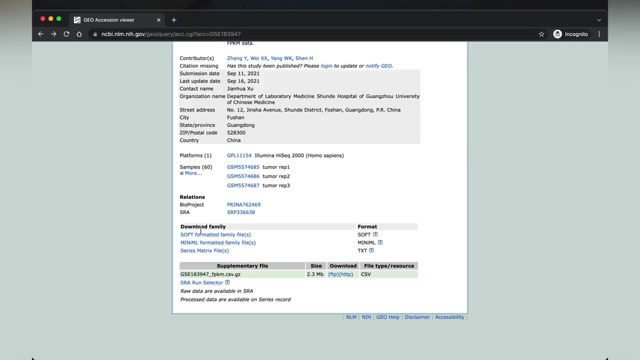 basically the sample was processed. The section following that we have links to some files- which has some metadata about this data set, which I'll talk about in more detail in my next video And in the last section. this is where we can find the gene expression data. Here we have our gene expression data with FPKM normalization. 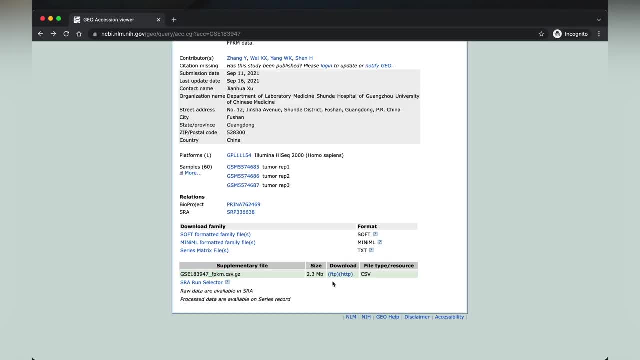 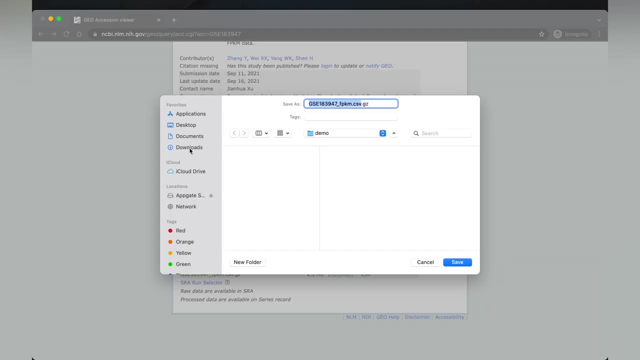 being performed and we have links to download it. We can download it using the FTP server or the HTTP. I'm going to use the HTTP, so I'm going to click on the HTTP and it opens a dialog box where it allows me to store this data to my local system. So I'm going to select the location where I want. 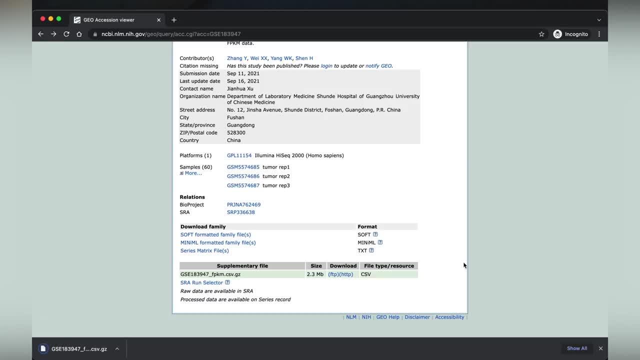 to save this data and I'm going to click on save As you can see that the data has successfully finished downloading. but I cannot open this file because you can see that there is a gz extension. That means that this data is gz compressed. 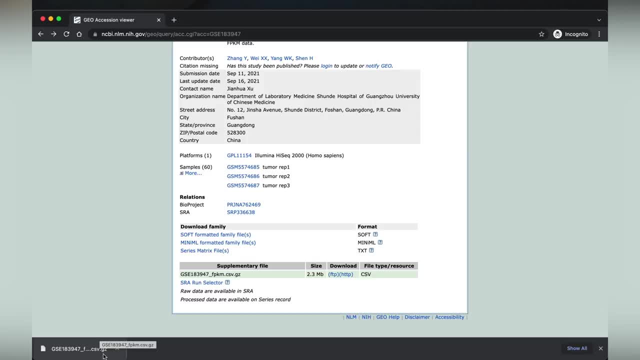 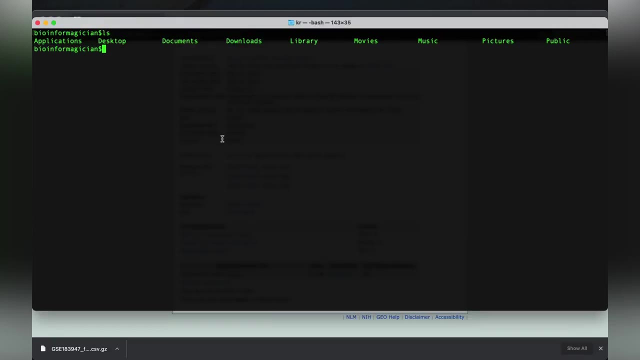 I have to first uncompress this file and then we will be able to see the csv file in Excel. To uncompress the gz file, I'm going to open my terminal. I'm just going to make it a little bigger so everybody can see that. 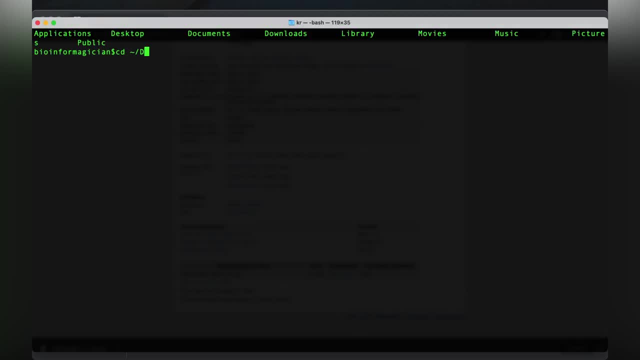 So this is my terminal and I'm going to go to the location of where I have stored my file. And when I list my file, I can see that this is where I have the file. And in order to uncompress this file, I'm just going to type in a command that's called gunzip and the name of the file. 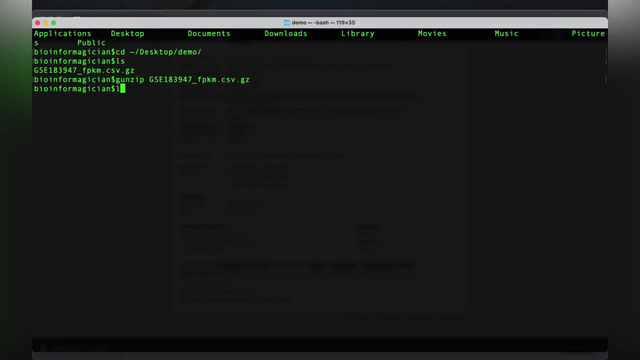 And I'm going to click on enter Once again. I will list my files and I see that the gz extension is no more present, which means that I can now open this file in Excel and can see the contents within. So let's go to our folder and open the file in Excel to see the contents within.